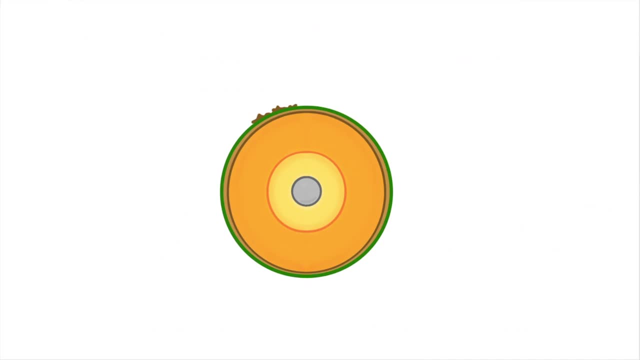 Like other waves, when seismic waves reach a boundary between two different mediums, they can be reflected, absorbed or transmitted And, importantly, when they're transmitted, they're often refracted, which means that they change direction And remember refraction. 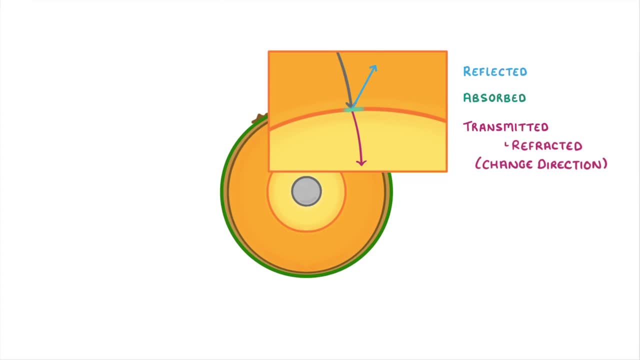 happens because waves change speed in mediums of different densities. At boundaries like this one between the mantle and the liquid outer core, there's a sudden change in density, and so there's also going to be a sudden change in the direction of the wave, Because the liquid outer core itself isn't all the same density either. 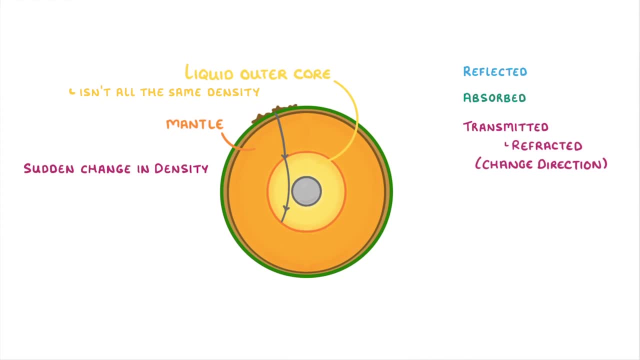 though, as waves pass through it, they're constantly being refracted slightly and so seem to curve as they slowly change direction. The same thing happens in the mantle, where it also isn't all the same density, And so, again, the waves are gently refracted and 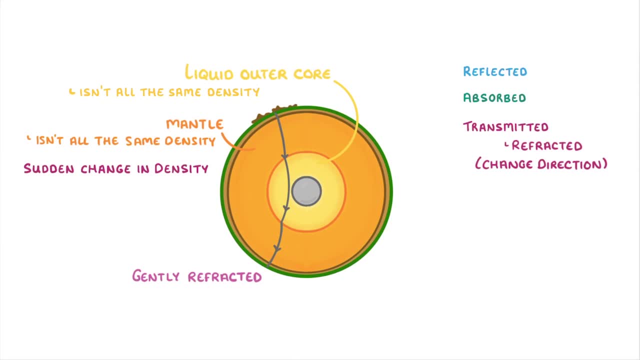 seem to curve. So if we did this for a whole bunch of waves, it would look something like this, with waves bending gradually while in the same section of the Earth, but more suddenly as they pass from one layer to another. Now, this diagram that we've drawn here is only true for P waves. 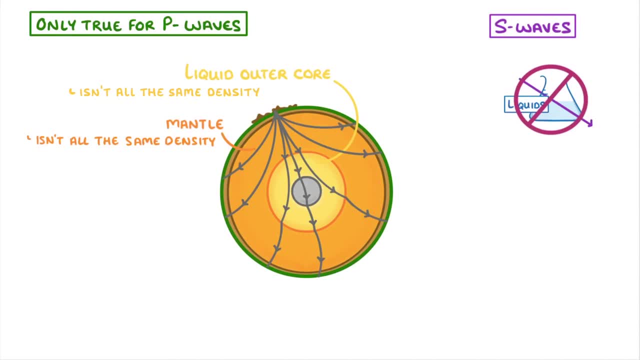 S waves, remember, can't travel through liquids and so can't pass through the liquid outer core. So instead of our lines going all the way through like this, they'd only be able to pass like this, And this was actually one of the main clues that led to scientists discovering 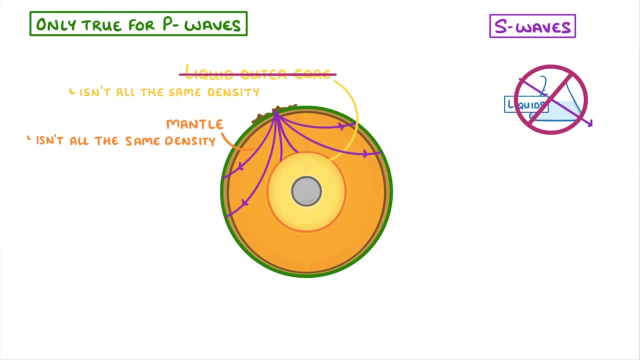 that we had a liquid outer core. The S waves could theoretically pass through the solid inner core, but they can't reach it because it's surrounded by the liquid outer core. This means that for our earthquake at the top of the Earth, S waves couldn't be detected. 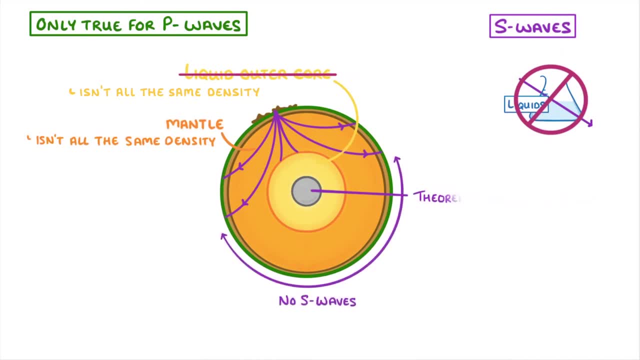 in any of this region, whereas P waves are detected almost everywhere. Oddly, though, they can't be detected at these positions, because any wave that passed through the outer core is refracted down here, and any wave that didn't will be refracted up here. So no waves.